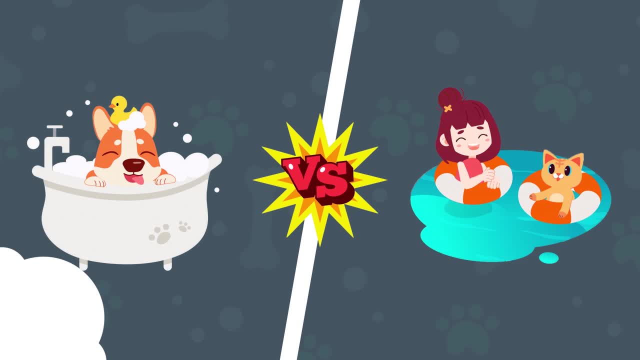 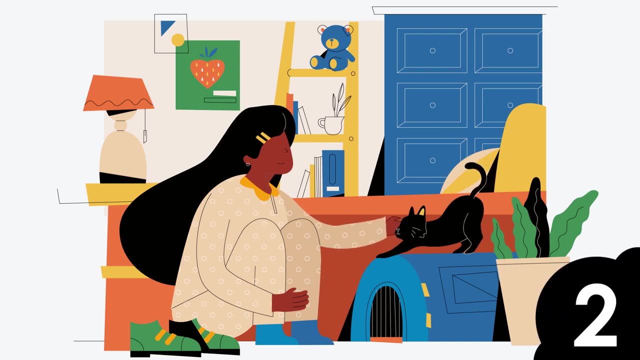 are trying to keep clean and odor-free, while a dog might smell bad. If that troubles you, you'd better think twice. Dogs are easier to train. Proud cats do whatever they want to. There is no easy way to know how a cat will behave. Cats think humans are the pets and not 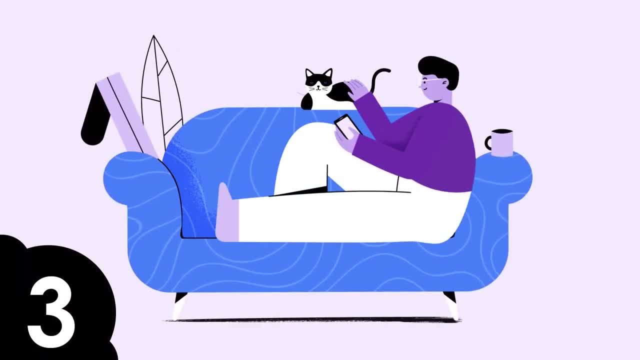 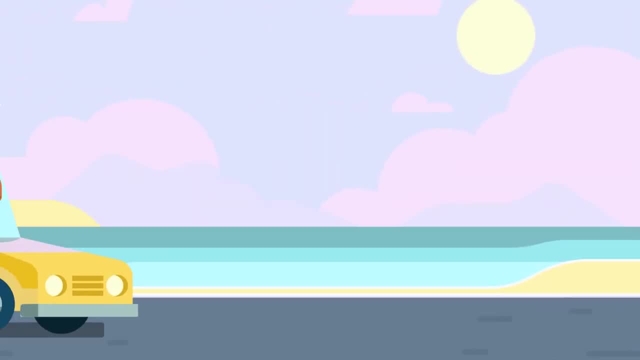 vice versa. Cats don't take up much space and are not so noisy. Nobody will run loudly around the house and wreck everything in its path. No animal can be more loyal than dogs. Your dog always follows you. Many people are saying that dogs are attached. 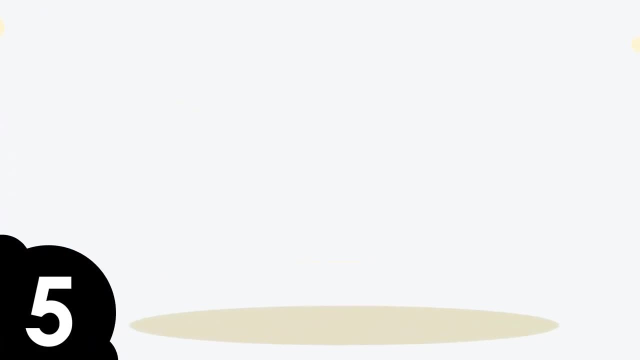 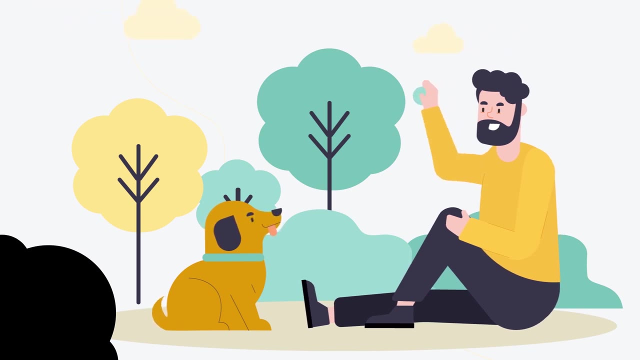 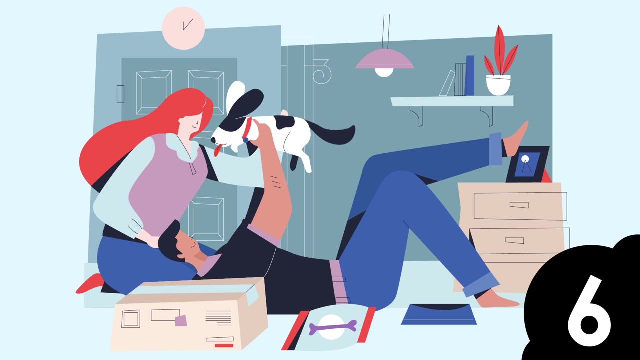 to a person and cats are more attached to their places. Every dog needs training and can learn commands, while a cat should be only taught to behave, to use a litter box and that's it. Dogs are a man's best friend. They comfort you every moment you have with them. There's nothing. 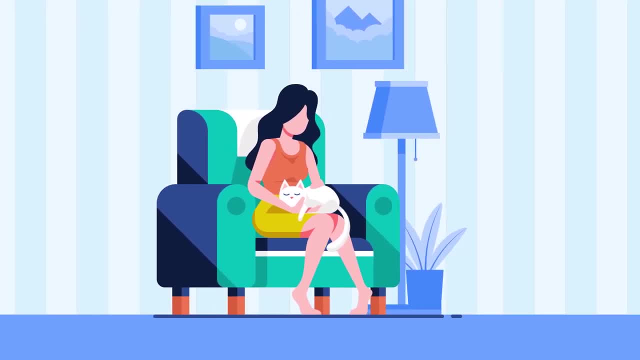 more important to your dog than your happiness. On the other hand, cats have a calming effect on your mind and soul. Cats purring is one of the most comforting sounds in the world. Pets are a serious financial undertaking so you need to budget. 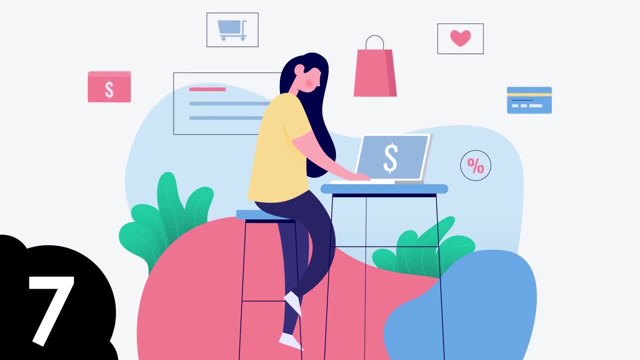 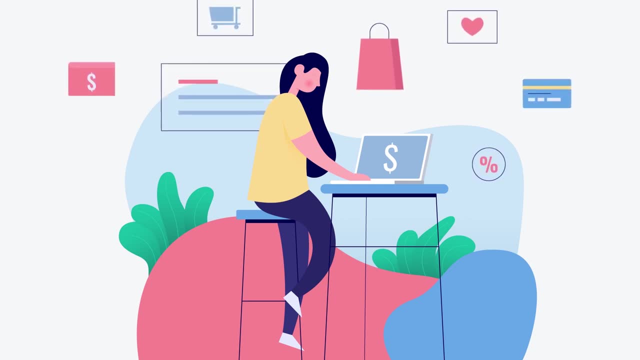 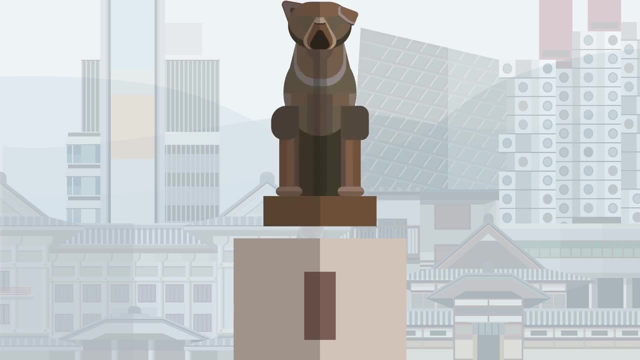 accordingly, You will need care products, toys, accessories and a bed, But it should be noted that a cat eats less food than even the smallest dog. For a dog, love for its master comes in the first place. We can see many examples of this in films and cartoons. Hachiko- A Dog's Purpose, Beethoven. 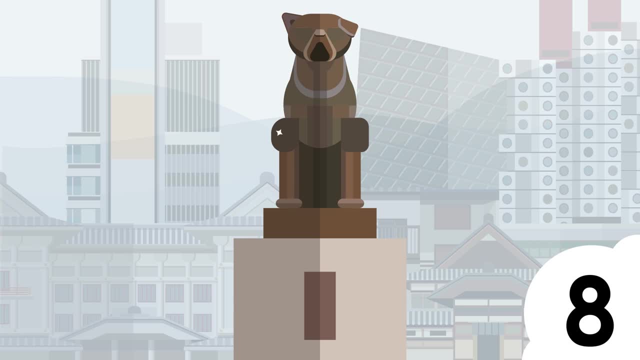 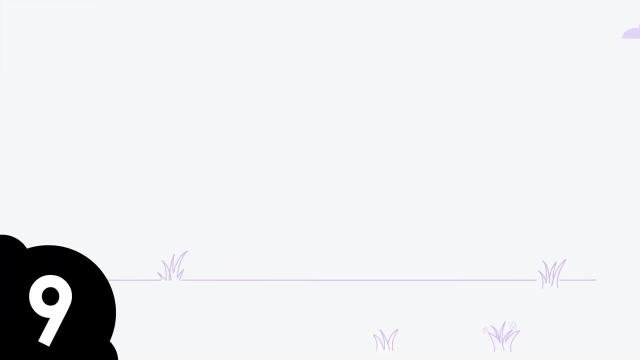 and many others. Cats are more selfish. They love you, of course, but less than themselves. Cats will communicate and play with you only if they want to. Some of them don't like being hugged and play with children, unlike dogs who are delighted to spend a lot of time with a human. Almost all dogs adore any child. they. 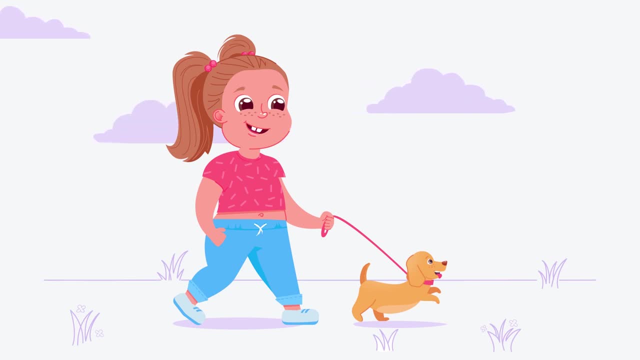 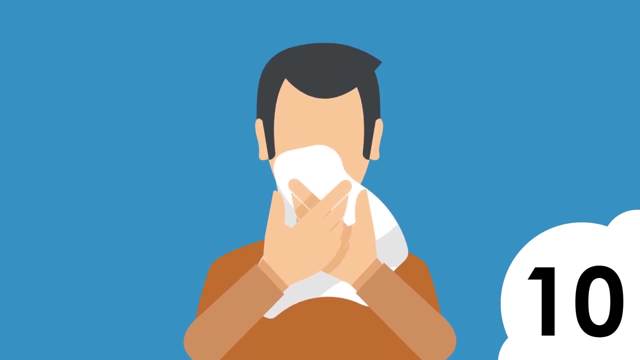 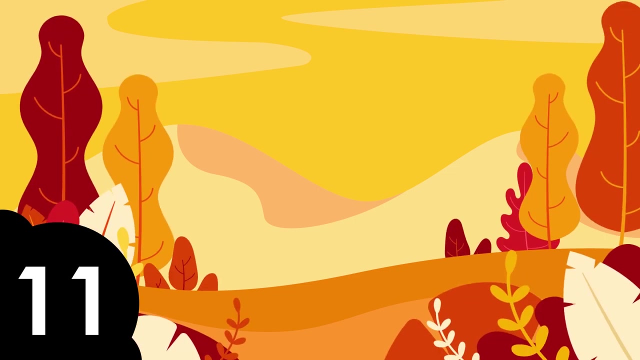 happen to meet and play Because our cat is indoor only. there's an excess of hair in the house that gets on furniture, bedding and clothes. Cats are more sensitive to the outside world than to the outside world. Cats don't need to be walked two to three times a day like a dog in any weather and